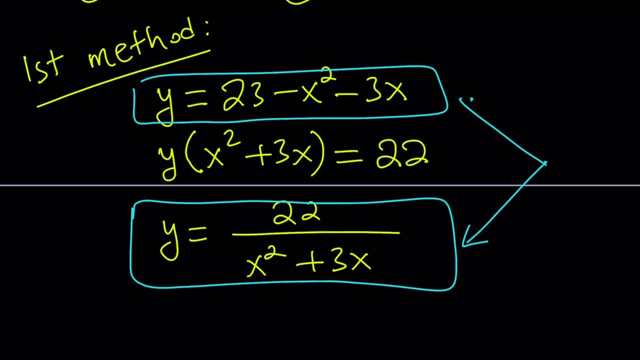 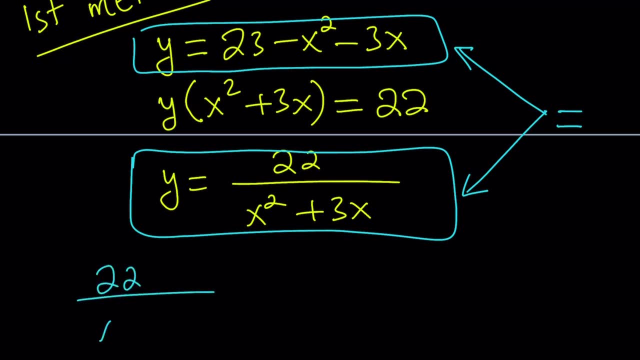 And since they're both equal to y, if two things are equal to the same thing, then they are equal, Right? so in other words, we can safely say that 22 divided by x, squared plus 3x, equals 23 minus x, squared minus 3x. Awesome, So here's what we can do. We can go ahead. 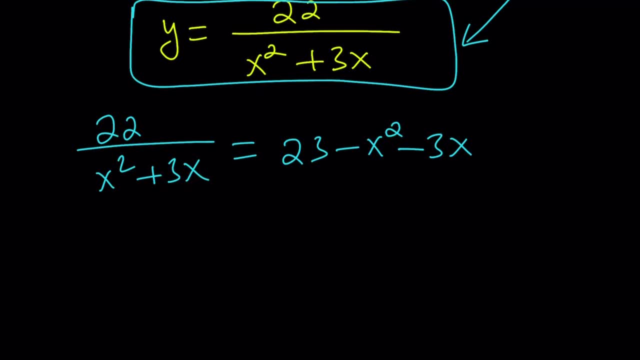 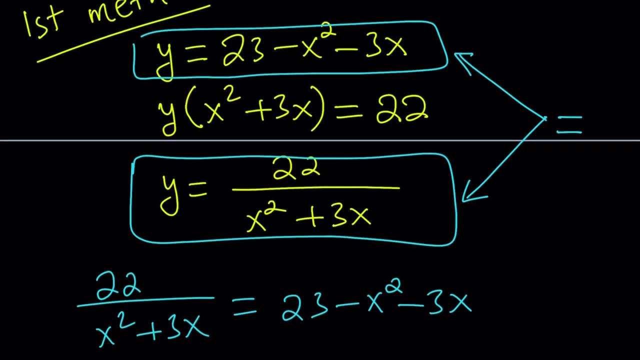 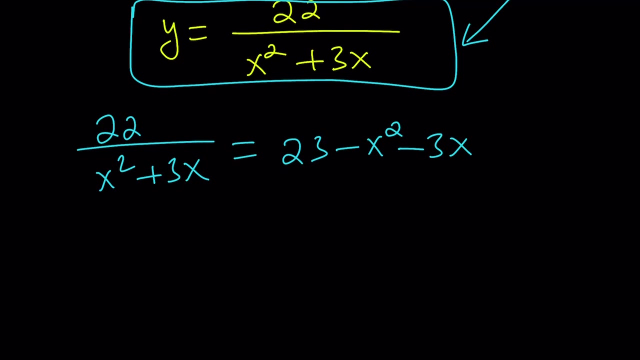 and cross, multiply and then put it all together and come up with a hopefully nice equation. It's not going to be that nice because this is the first method. Obviously the second method will be nicer and I can clearly think of a third method which is kind of similar to the maybe not second. 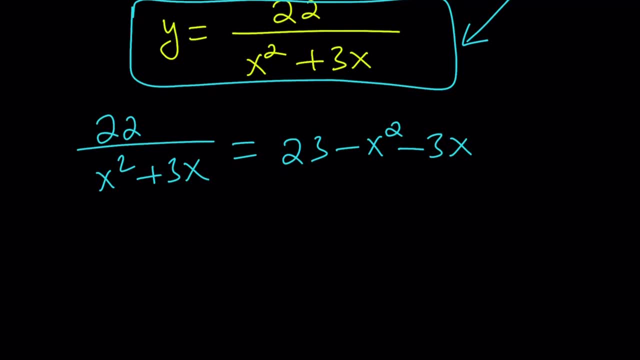 but kind of first. Anyways, let's just stick with two methods here. So if you cross multiply, you're going to get 22 equals x squared. Let's go ahead and distribute the x squared first: 23x squared minus x squared. 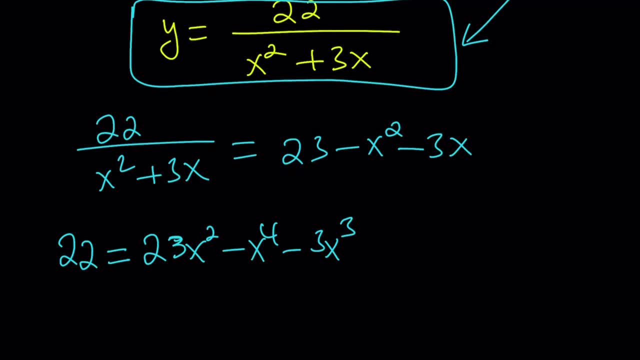 minus x to the fourth, minus 3x cubed, And then let's distribute to 3x plus 69x, minus 3x cubed minus 9x squared, I have x to the fourth. Let's put everything on the left hand side so that x. 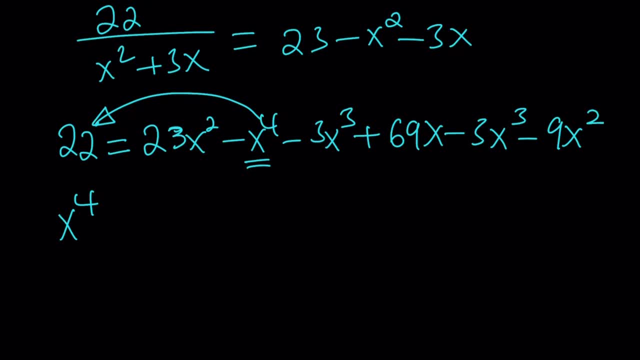 to the fourth becomes positive. So we have x to the fourth, And then I have negative 3x cubed. negative 3x cubed makes 6, negative 6, but on the left hand side that's going to be a positive. 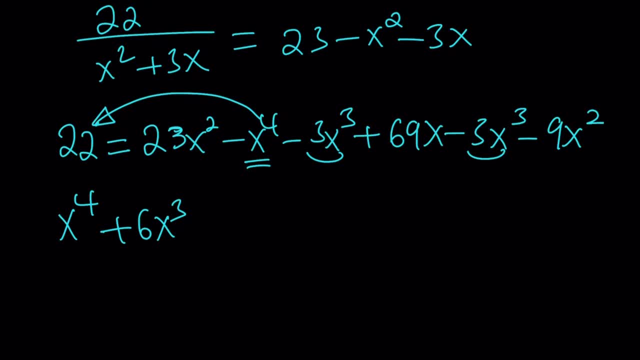 6x cubed. And then I have some x squared right: 23 minus 9 is 14, but that's going to be negative 14 on the left hand side. And then finally we have the 69x which we can subtract and get. 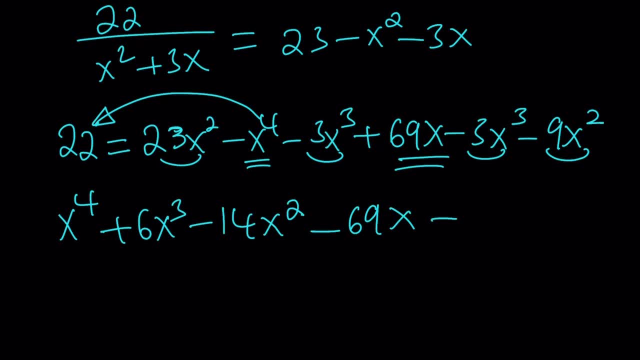 negative 69x. And, of course, we already have our constant there, 22,, which is just going to stay there. Awesome, Well, not so awesome because, come on, this is a quartic equation. Do you seriously want to use the quartic formula, which is: 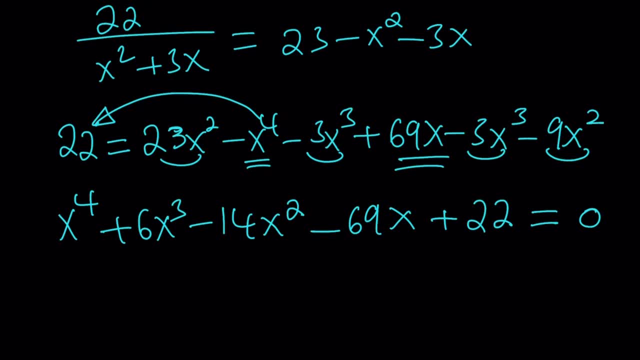 super, super complicated, But with certain methods, you know, you can just go ahead and turn this into a cubic equation and then solve that cubic equation by using some method which was invented by some Italian guy, and then so on and so forth. right, Okay? So anyways. 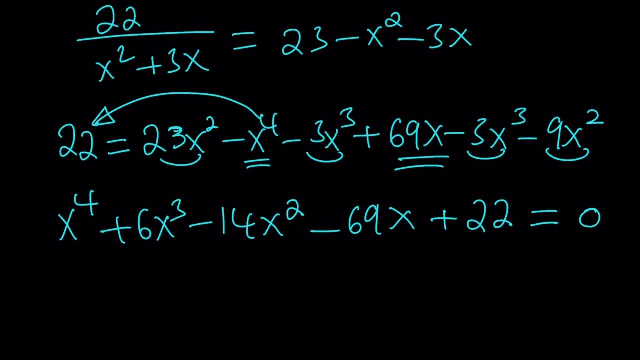 one of the things we can possibly do is if x is an integer, then hopefully it is, but it may not be. we can go ahead and kind of use rational root theorem. If one of the roots is rational, then we can use the rational root theorem. So if one of the roots is rational, 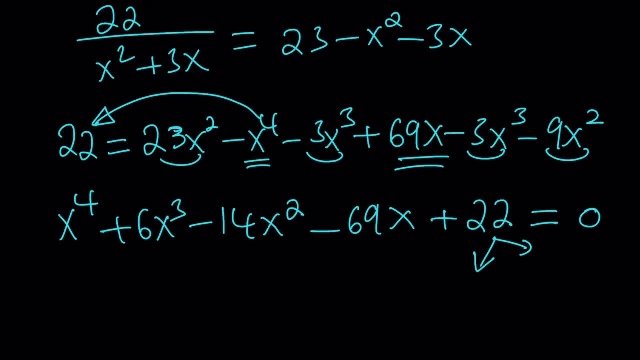 we can kind of look at divisors of 22 or factors which are potential candidates, So kind of like plus minus one, plus minus two, plus minus 11,, plus minus 22.. So those are the candidates. Good luck with that. And then they may not work at the end, right? So if that doesn't work, 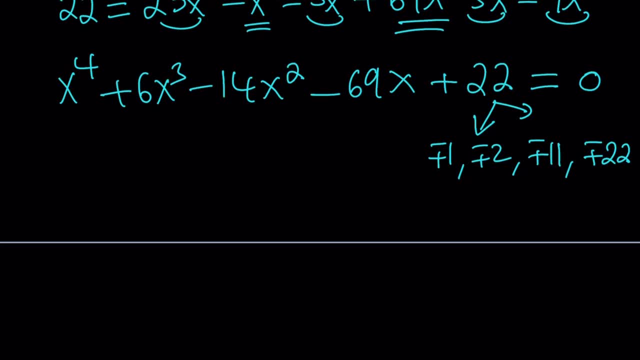 we can also try to factor this, But one of the things we should probably do is get rid of the x cubed first and then write this into like kind of like a product of two quadratics. I think it's called Descartes. 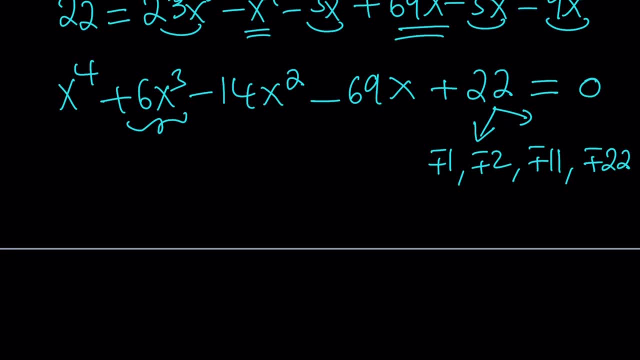 method or something like that, I don't know. Can you remember that? So basically, get rid of. to get rid of the x cubed, you should replace x with something like y minus. So here's what you need to do: Divide the coefficient of x cubed by the highest power, which is four, and put a minus. 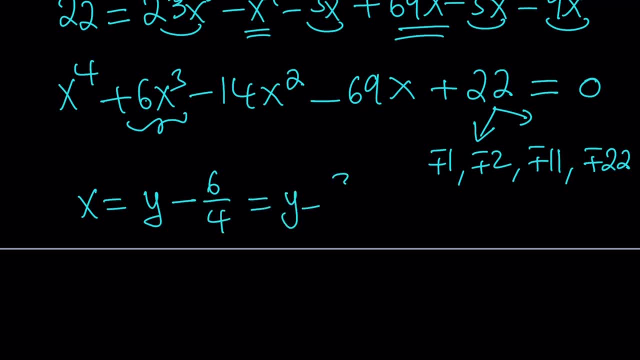 sign. So it will be this And obviously this is not going to be that nice. So you're going to be dealing with a lot of difficulties, especially with fractions, so on and so forth. So that's super painful. Hopefully you see that. 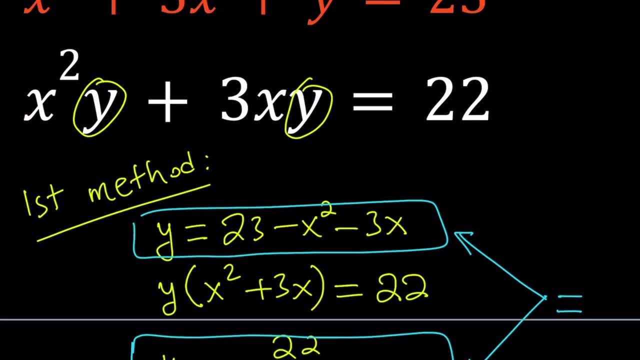 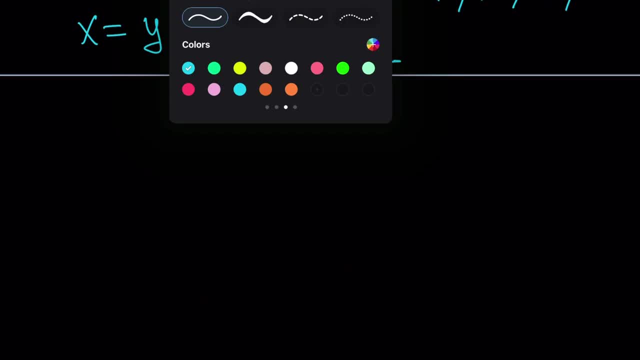 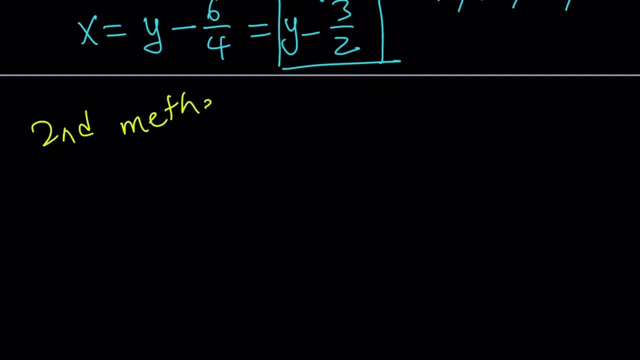 method is not very elegant, right, And there's a reason why. there's a second method which is much more elegant, And let's talk about that. And of course, after the second method we can kind of go back and revisit first method and see how we could proceed a little differently to make things. 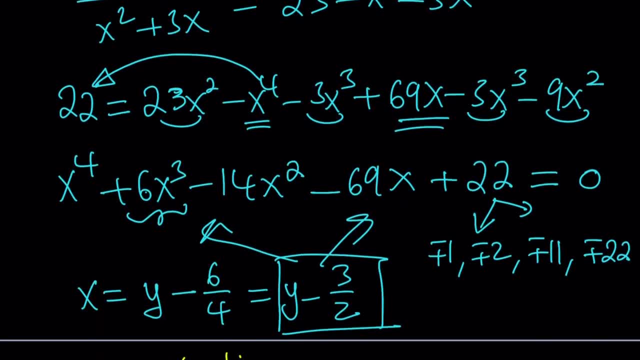 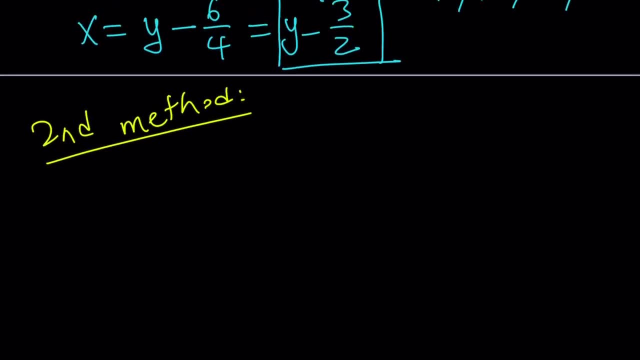 easier. I know what you guys are. some of you, some of you are thinking, hey, why didn't you do this, Why didn't you do that? I deliberately avoided some of the easier paths. Okay, Forgive me for that, All right. So here's what we're going to do. to proceed, I'm going to rewrite my system. 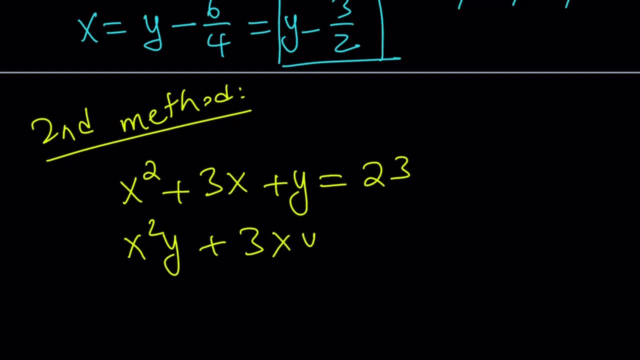 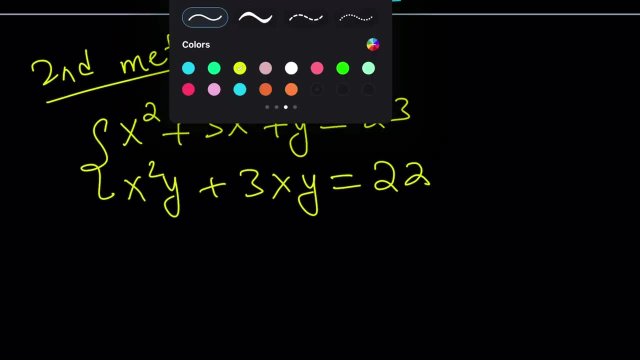 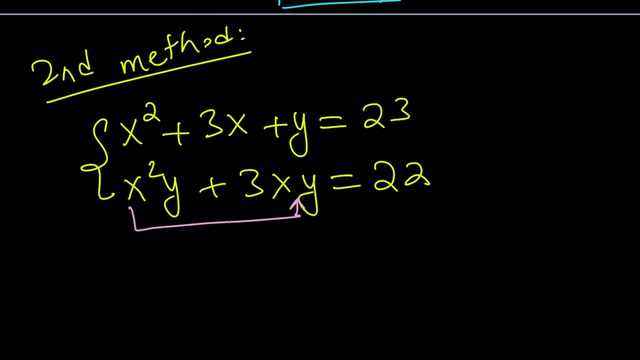 And then I'm going to manipulate this a little bit to get what I want, because this problem is, as some people say, contrived, Okay, So how do you get the trick? So here's the trick. First of all, I noticed that I can take out an X- Y here. Let's do it: If I take out X- Y, I end up. 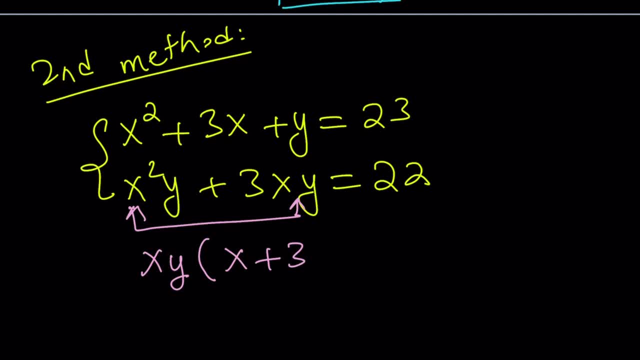 with X plus three. That's it: X plus three. That's it right. Okay, good, I was expecting to get more terms, but that's it Anyways. so I get this And from the second equation. here's what I can do: I. 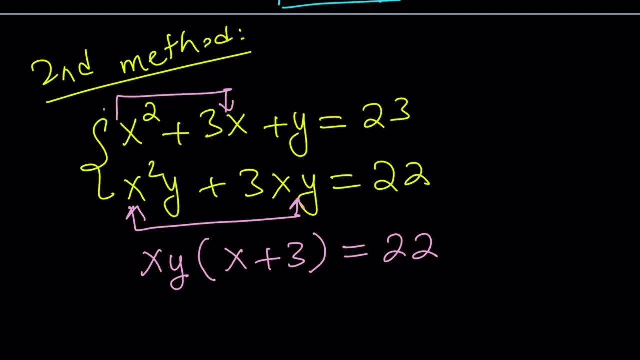 can't completely factor it, but I can take these two terms and factor out an X and write it as: X times plus 3 plus y equals 23.. So this is my new system, And guess what This is actually in. really good. 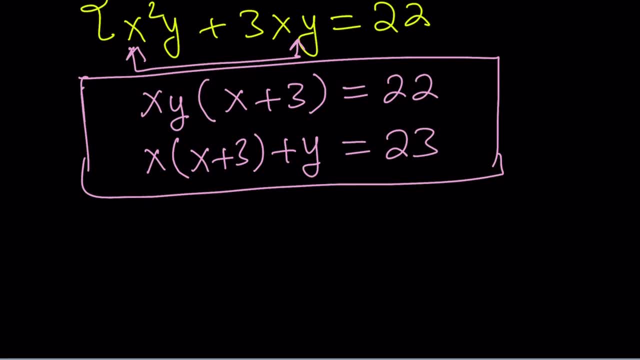 shape. I'll tell you why in a little bit. So if you go ahead and do the following, Put the x and x plus 3 together. Now here's what's going on. Let me tell you Here's a trick. Notice that x times. 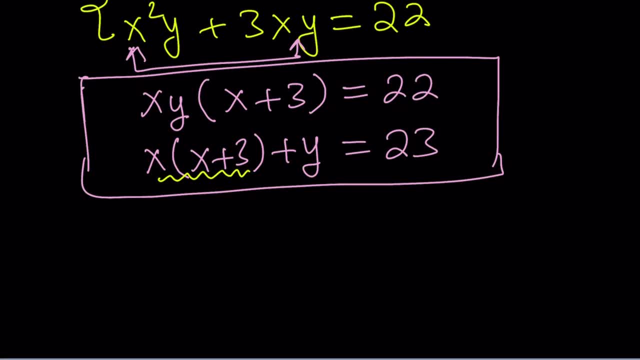 x plus 3 is kind of like together. Then they make up an entity And then y is being added. So if I put these two together, then I'll be getting the same thing. So let me rewrite my equation that way: x times x plus 3 times y equals 22.. x times x plus 3 plus y is 23.. Hopefully you see what I see. 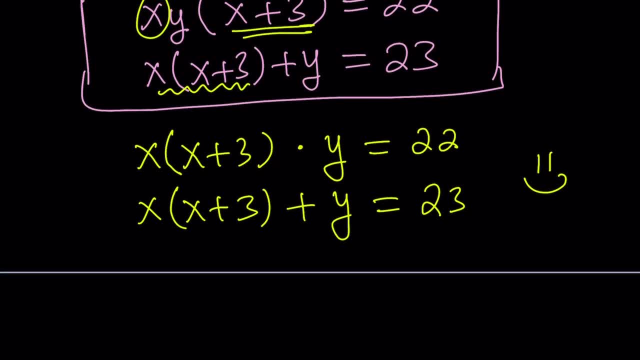 And if you do, here's what I'm talking about. Let's call this x times x plus 3 thing. another variable like z, And we can stick with the y Because it's already a good variable. right, y is a good variable, So from first equation, this is also z. 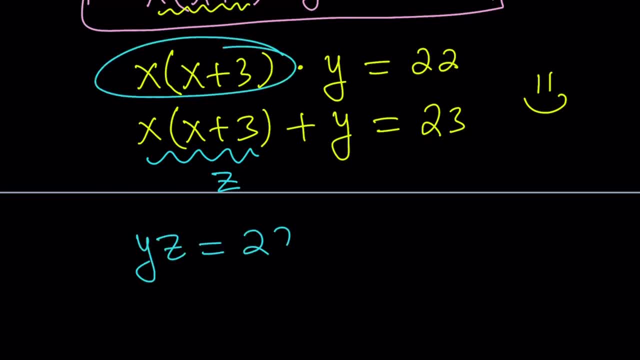 by the way, First equation gives us y z equals 22.. I'm kind of obsessed. I need to write everything in alphabetical order most of the time, And then y plus z is 23.. This is one of the nicest systems that you can get, besides y plus z and y minus z, which is never going to happen, by the way. But 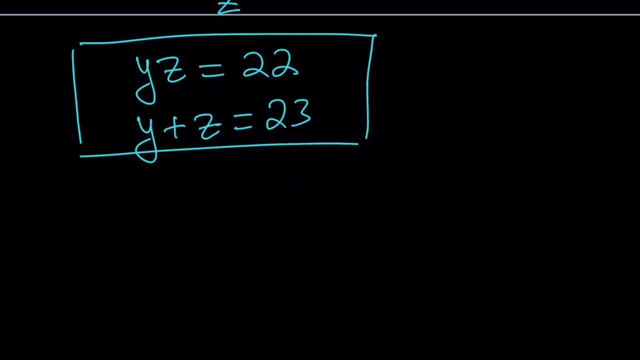 anyways, this is pretty easy. Now you're thinking, hopefully finding two numbers, whose product is 22.. And whose sum is 23.. And guess what? Those numbers are 22 and 1.. And, of course, vice versa. Great, This is awesome, isn't it, Don't you think? So we got the y value right away, Or y is 1 and z? 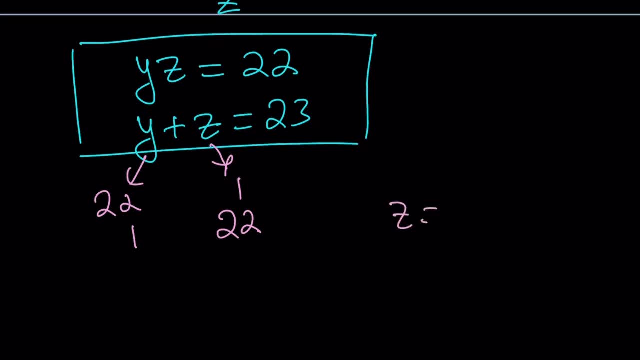 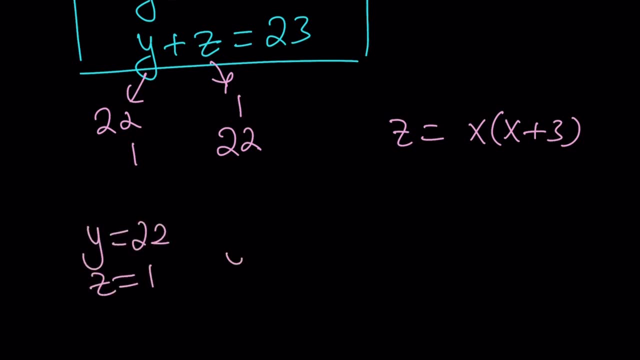 is 22.. But what is z? z is x times x plus 3.. So we get the following system: y is 22,, z is 1. Or y is 1,, z is 22.. And again, this is super duper awesome Because I got. 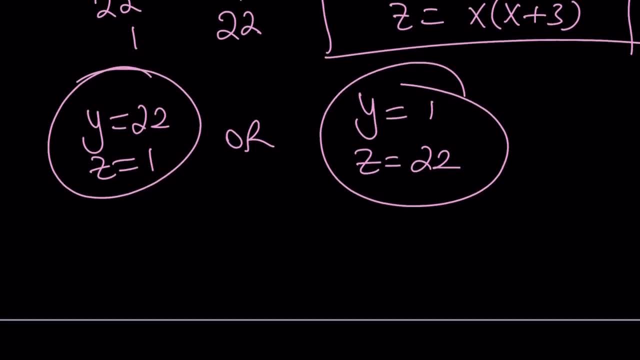 z here, And let's go ahead and write our equation one more time. We got y equals 22.. That gives us the value of y right away. But we also got x times x plus 3 equals 22,, which gives us x squared plus. 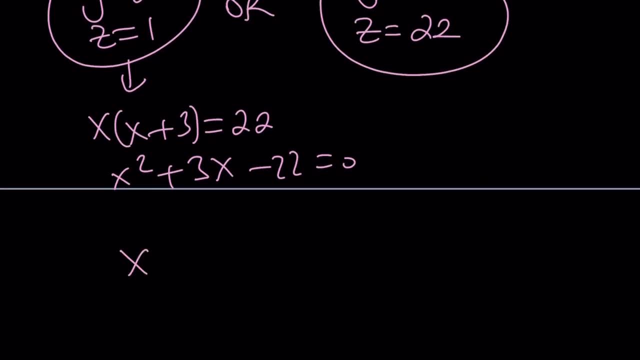 3x minus 22 equals 0. And from here x equals negative b plus minus the square root of b squared, which is 9, minus 4ac plus 88. And that's not going to be a super duper nice answer. But 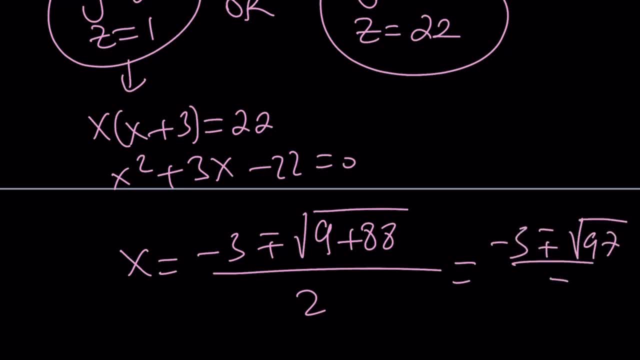 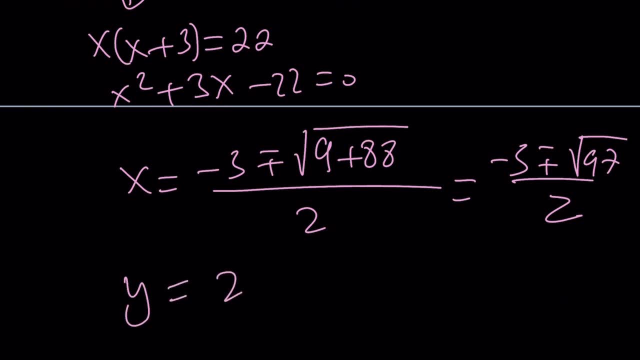 guess what That's going to work? Okay, So those are the x's and y's And we're going to write our x values: for y equals 22. And if y is equal to 1,, this is: for y equals 22.. And if y is equal to 1: 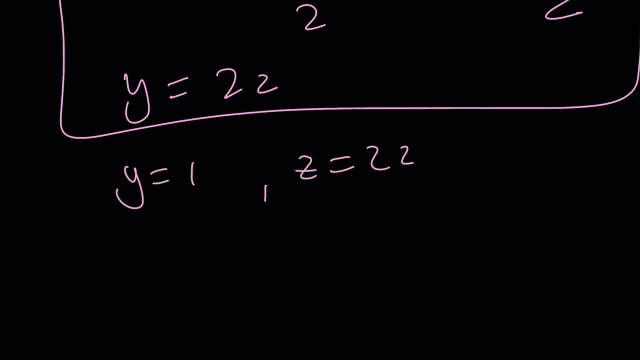 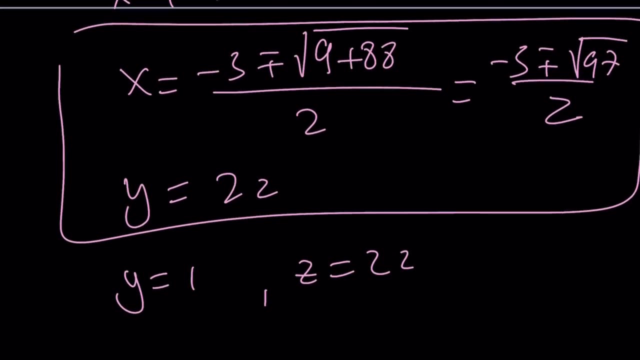 and z is equal to 22,. then we get the following: Because x times x plus 3 is- wait a minute, I think I messed up. Y is 22,. y is 1.. Okay, Y is 1.. So y is 22.. Okay, I messed up on this one. 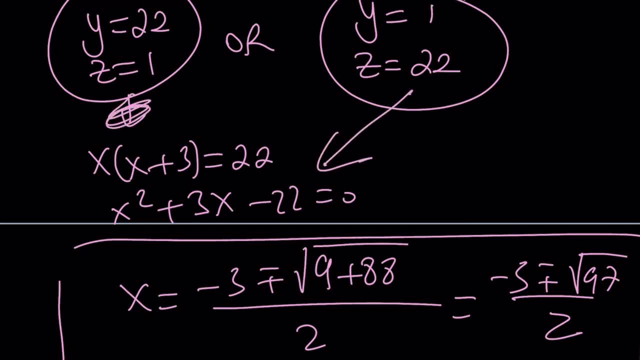 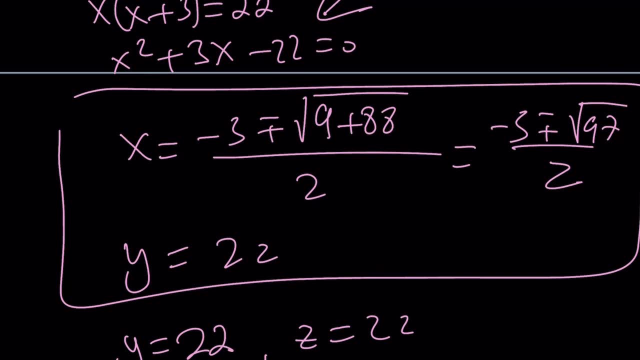 This belongs to the other one. Okay, Here we go. It's for this one. Now we're doing: y equals 22 and z is 1.. Y is 22 and z is 1.. Sorry about that, And in this case we get x times x plus 3. 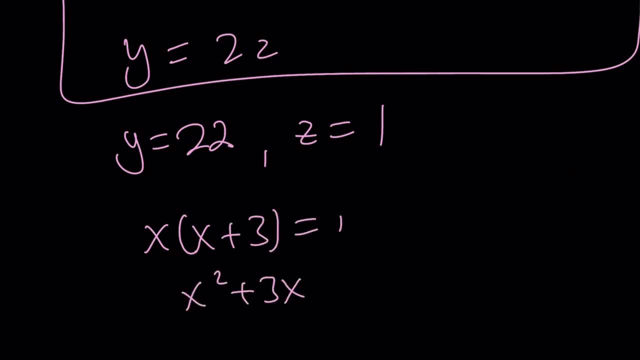 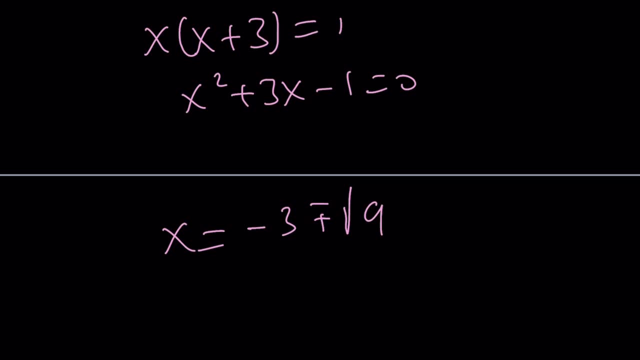 equals 1,. x squared plus 3x minus 1 equals 0.. And from here we get: x equals negative 3 plus minus the square root of b squared minus 4ac, And that's going to give you square root of 13.. And that's.